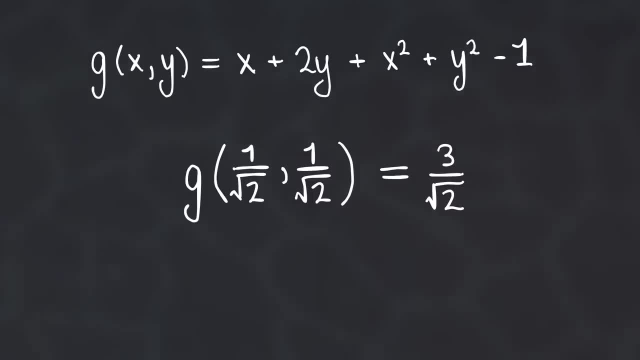 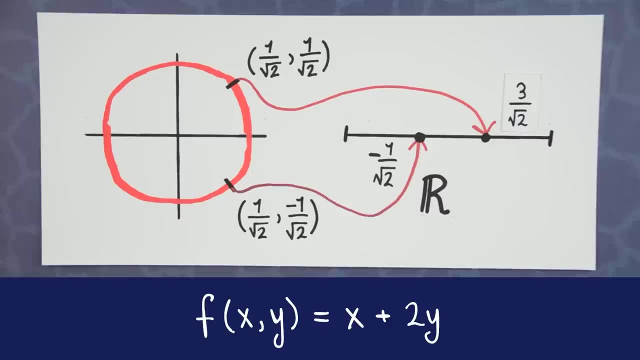 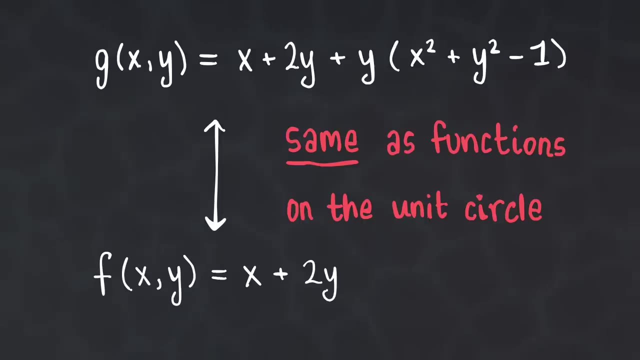 g is 3 over the square root of 2, and g of this point is minus 1 over root 2.. Notice that these are the same outputs produced by our function f from earlier. The same will be true for these two functions. They are the same as functions on the unit. 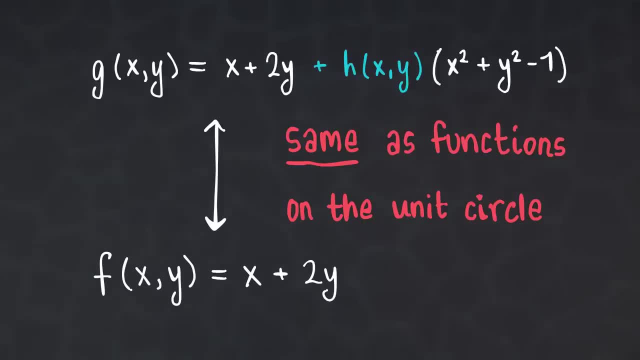 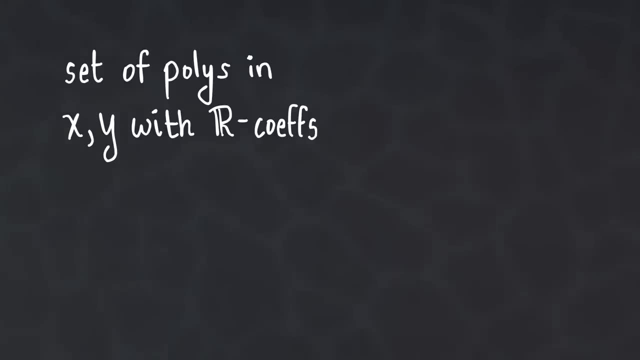 circle. More generally, any function of this form will be the same as f. Let's phrase this in a more sophisticated language: The set of polynomials in the variables f and g are the same as functions on the unit circle. The set of polynomials in the variables f and g are the same as functions on the unit. 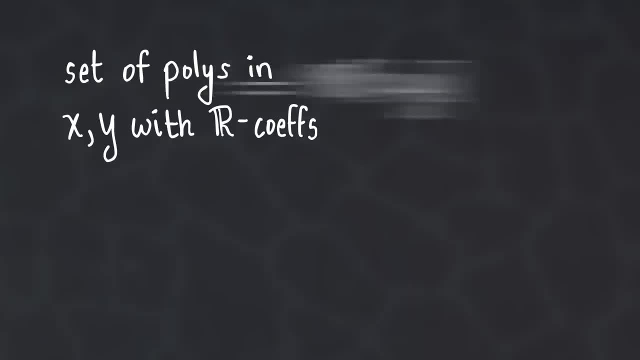 x and y with real coordinates is denoted r, bracket x, comma y. this is more than just a set. it's closed under addition. if you add two polynomials with real coefficients, you get a polynomial with real coefficients. it's also closed under multiplication, an algebraic object. 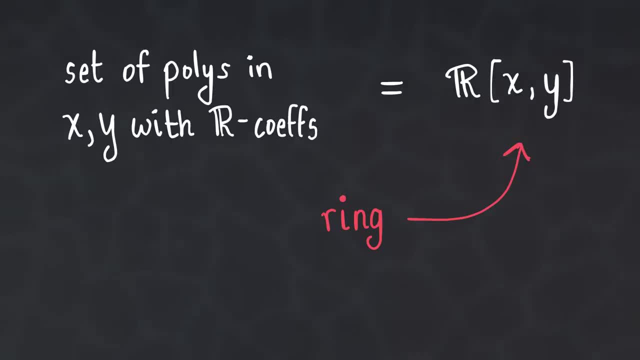 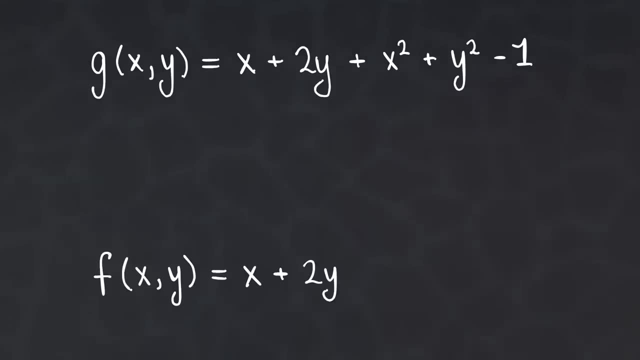 that behaves in this way is called a ring. now look at the set r of all polynomial functions defined on the unit circle. we think of two polynomials as defining the same function. if they agree on all points- x, y- on the unit circle, then they are equal as members of r. we can add and multiply. 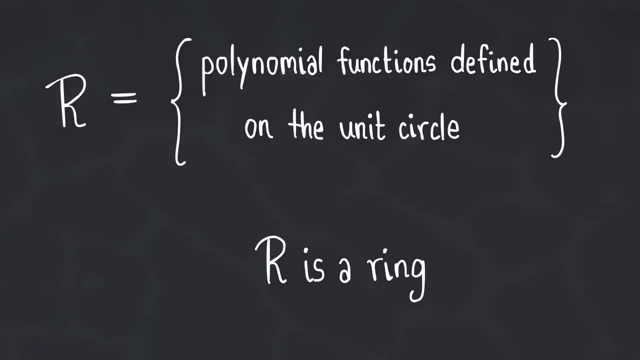 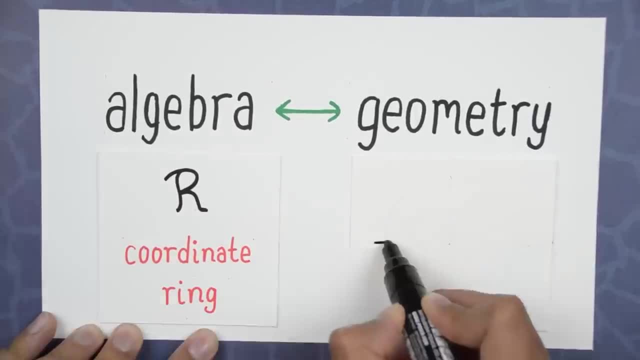 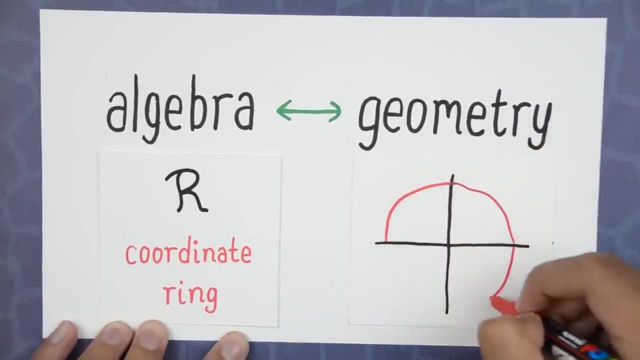 functions in r. therefore r is a ring, some terminology. this ring r is called the coordinate ring of the circle. we view it as an algebraic manifestation of the circle. as we will see, geometric properties of the circle are encoded in the algebraic properties of its coordinate ring. 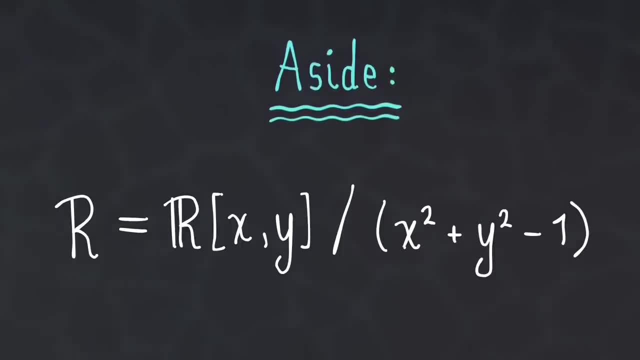 a small aside: for those who know some ring theory, you'll realize that what we're doing here is working with the quotient ring of r bracket, x, y modulo, the ideal generated by x squared plus y squared minus one. now, if those words don't make any sense, don't worry about it, we won't need it. 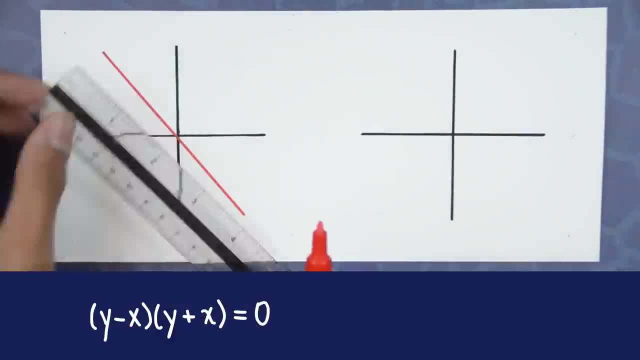 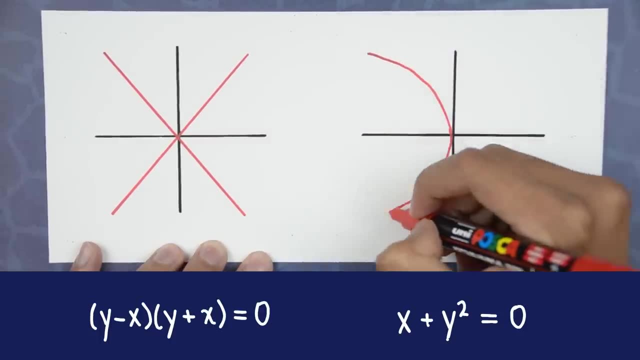 for the rest of the video, look at this curve: y minus x times y plus x equals zero. versus this parabola: x plus y squared equals zero. the first curve is a union of two curves and the second one isn't. we say that this curve is reducible and this curve is irreducible. 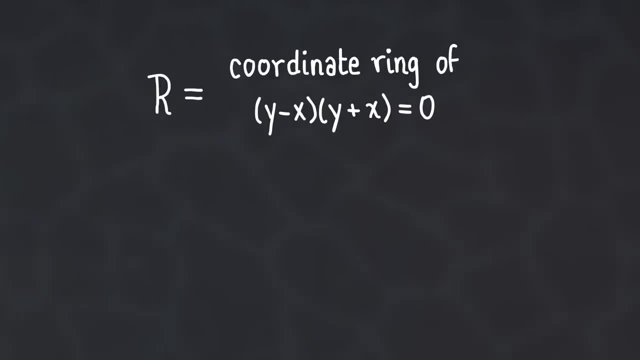 let r be the ring of functions of the first curve and let s be the ring of functions of the second curve. the algebra of these two rings, as we will see, is quite different. the first ring, r, is kind of weird. consider the function f of x. y equals y plus x squared plus y. 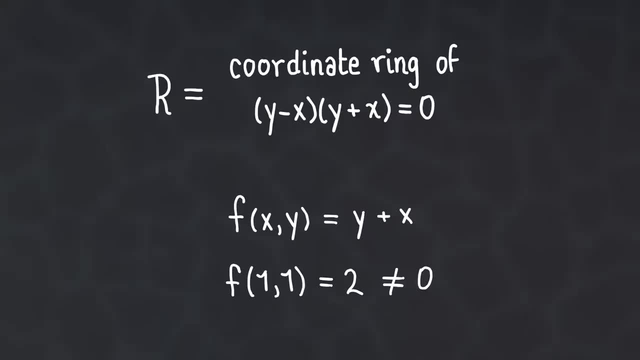 plus x. in R, It's not identically zero. For example, f is equal to 2, and this is clearly non-zero. Similarly, the function g equals y minus x is not zero on the curve either. However, the product is zero on all points of the curve. This type of behavior might 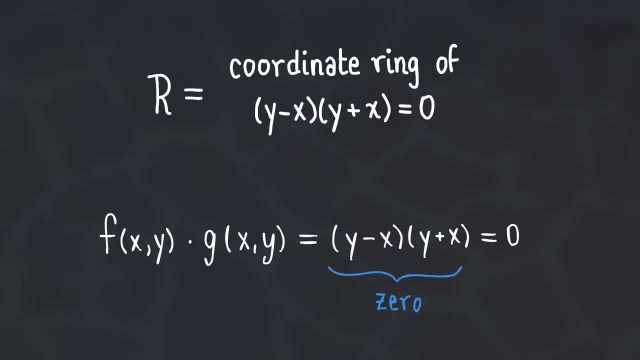 feel strange. The product of two things is zero, but both of the factors are non-zero. This never happens in the ring R. It turns out- and this is not immediately obvious- that if the product of two polynomials is zero on the parabola, then at least one of 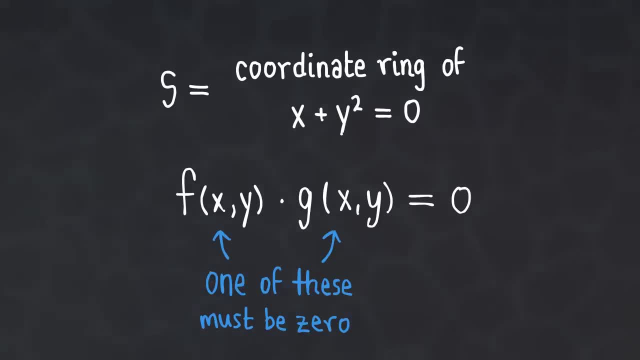 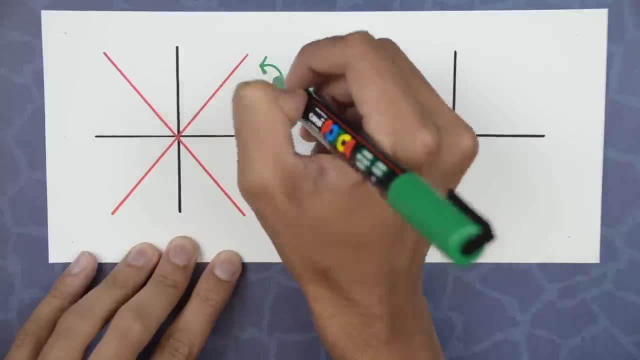 the two factors must be zero on the parabola. This algebraic phenomenon is detecting that the first curve has two pieces- it is reducible, while the second curve has only one piece- it's irreducible. The geometry of whether the curve is irreducible or not is appearing. 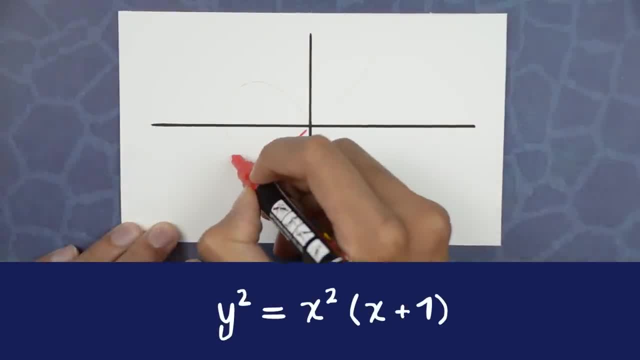 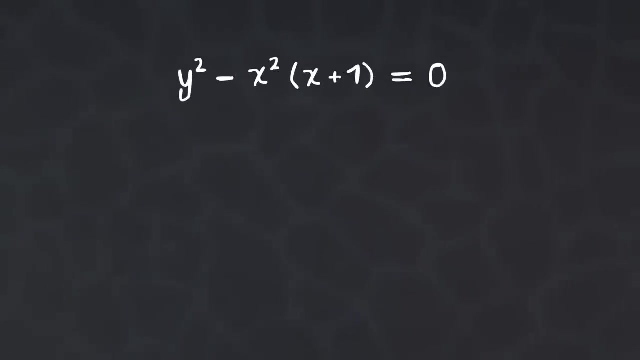 in the algebra. Here's a more complex example. The curve y squared equals x squared times x plus 1.. This curve intersects itself. It has a node at the origin. Can we detect this using algebra? First, let's bring all the terms to one side, Using the formula for a difference of squares. 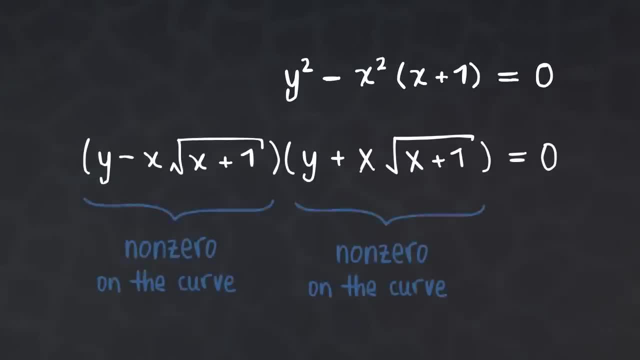 let's write this as follows As before. notice that these two functions are both non-zero on the curve, but the product of these two functions is zero on the curve If you zoom into the origin. the function g equals x squared times. x plus 1 is not zero on the curve. 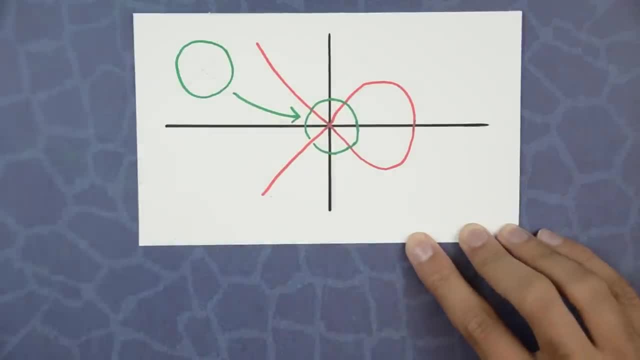 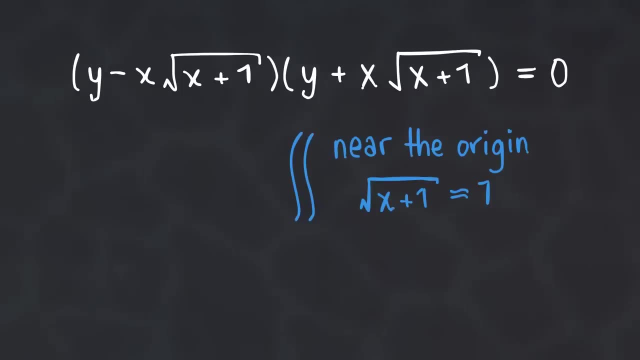 Notice that these two functions are both non-zero on the curve, but the product of these two functions is zero on the curve. This looks like two lines crossing each other. So near the origin. this curve look is reducible Algebraically. near the origin, square root of x plus 1 is approximately equal to 1.. 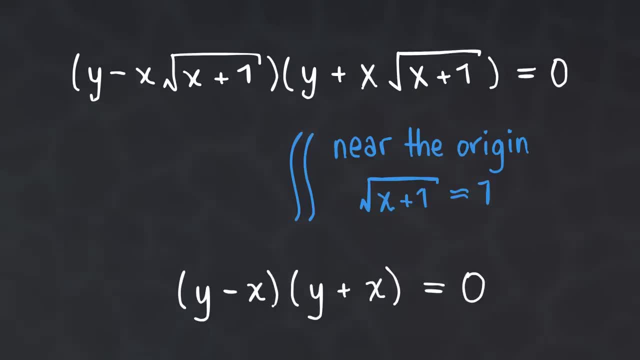 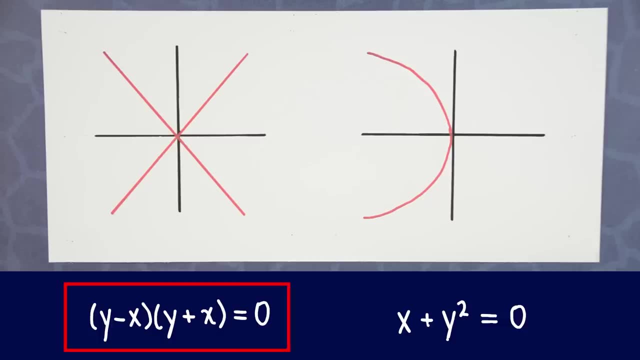 so this top equation is approximately equal to this bottom equation And the bottom equation, if you'll remember, was precisely the equation of the two lines crossing each other from before. But there is a problem: up until now we have only been looking at polynomial functions. 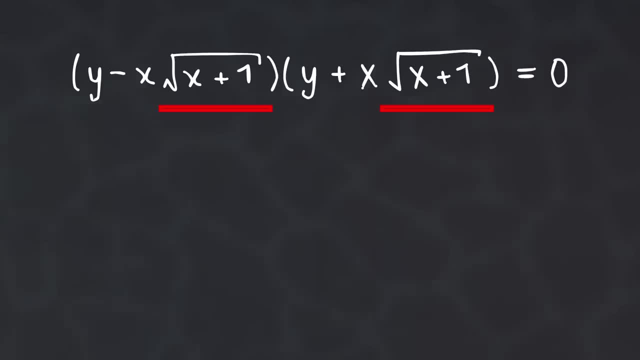 But the square root of x plus 1 is only zero, and the square root of x first is zero. 1 isn't a polynomial. what ring does the square root of x plus 1 live in? well, the secret is to use a tool from calculus. we can write the taylor series of the square root of x plus 1 as follows: 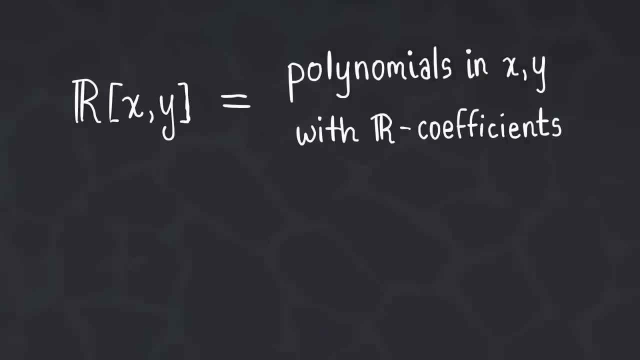 previously we looked at the polynomial ring r of x- y. now we're going to look at a power series, ring r, double bracket x- y. this is defined as a set of all formal power series in x comma y with r coefficients. we will think of the function, the square root of 1, as belonging to the power series. 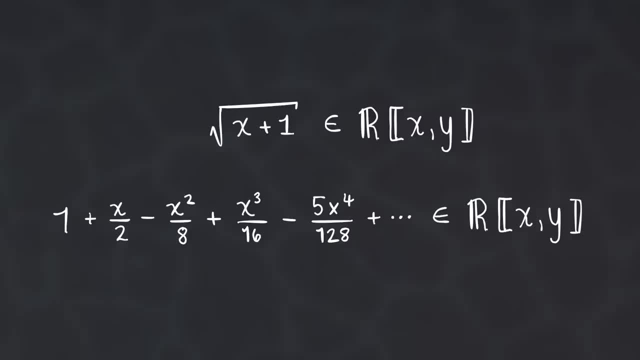 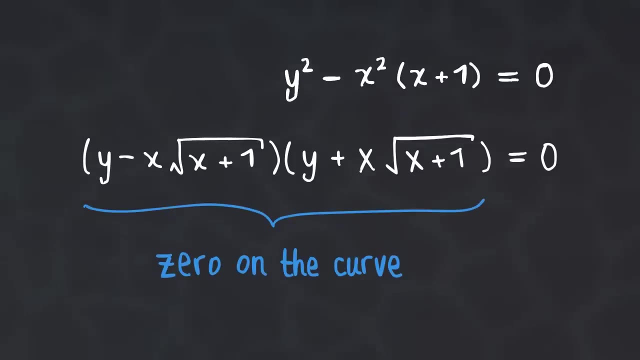 ring r, double bracket x, y, or more precisely its taylor expansion, belongs to this power series ring. so what we've noticed is that there are formal power series which are individually non-zero on the curve, but the product of them is zero on the curve. this detects the fact that 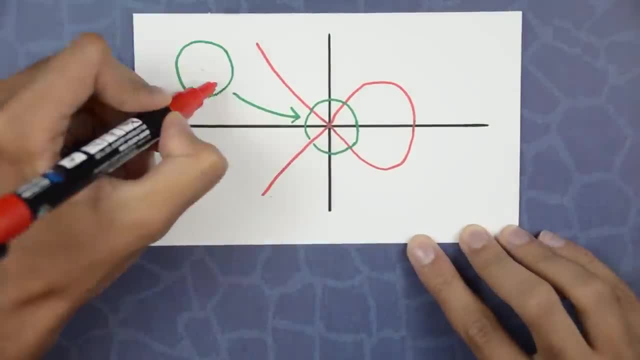 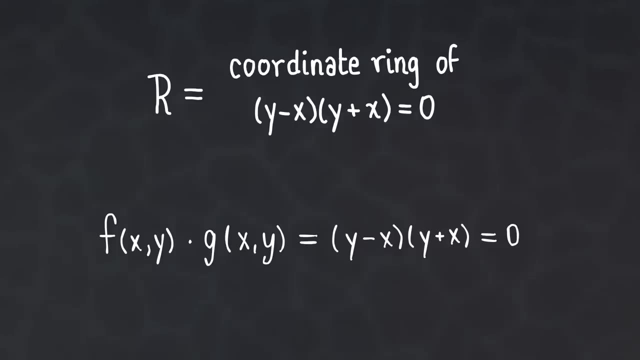 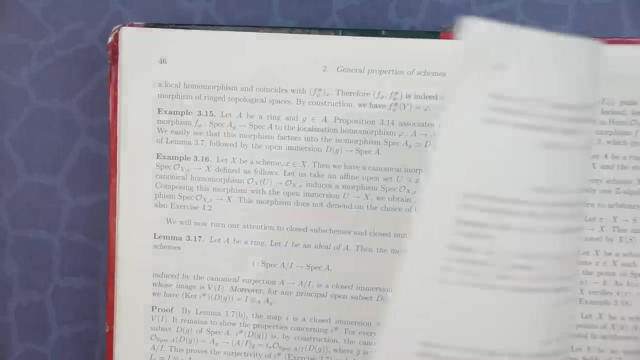 if you zoom into the origin, the curve has two lines that look like they're crossing themselves. but who cares about the algebra geometry dictionary that we've been talking about? well, the benefit of this is that algebra helps us nail down geometric intuition into rigorous math. this is why, if you look at most textbook and algebraic geometry, most proofs use ring theory. 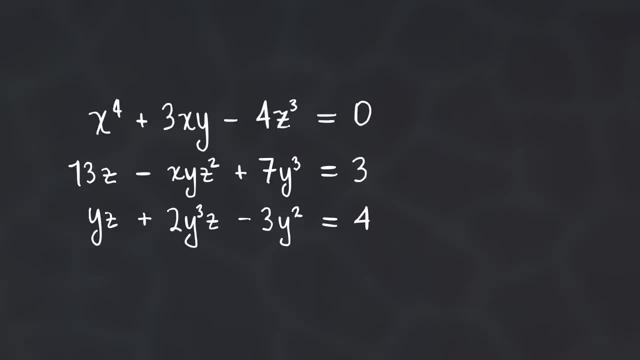 quite heavily. furthermore, if i give you a shape that's carved out by these three polynomials and i ask you: what are the singular points? is it irreducible? i mean, you can't visualize it and tell me the answer. but you can't visualize it and tell me the answer, but you can't visualize it. 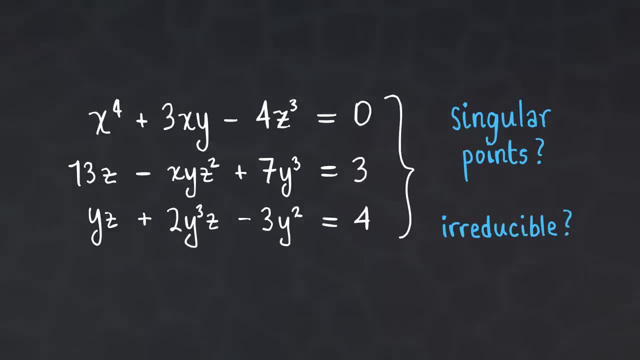 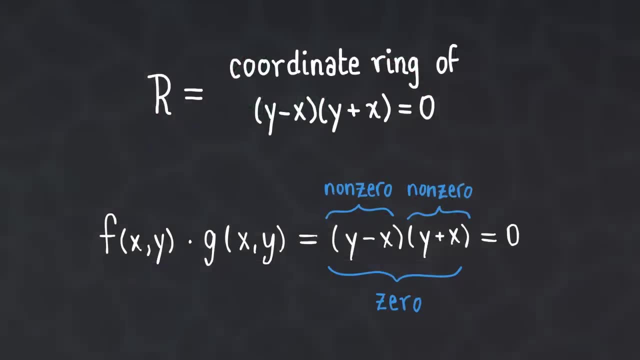 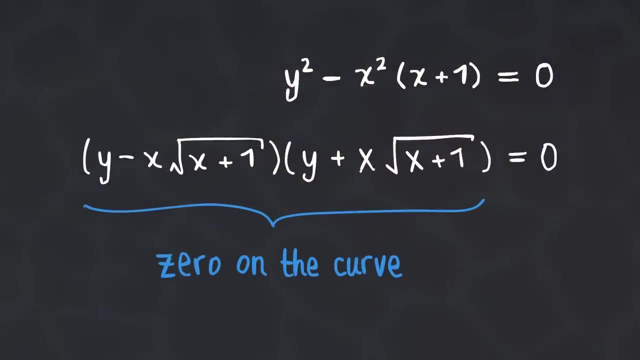 but you can compute its coordinate ring and tell me its properties. so far, we've seen two geometric properties of curves that are captured by their coordinate rings: irreducibility, and a curve having a node. the takeaway of this is that we can translate geometric phenomena into algebraic properties. 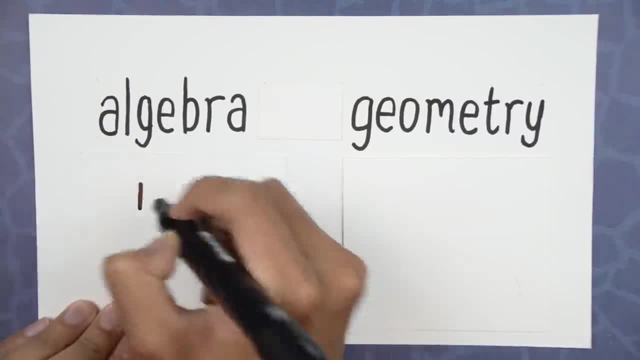 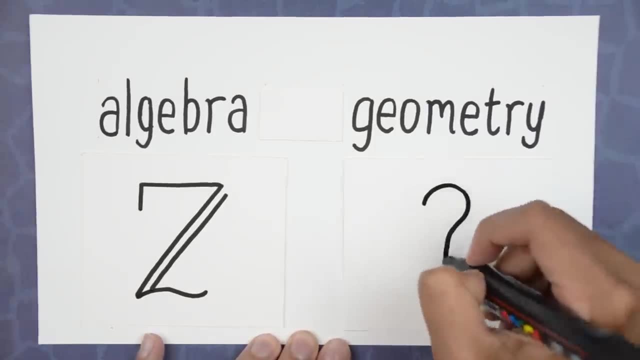 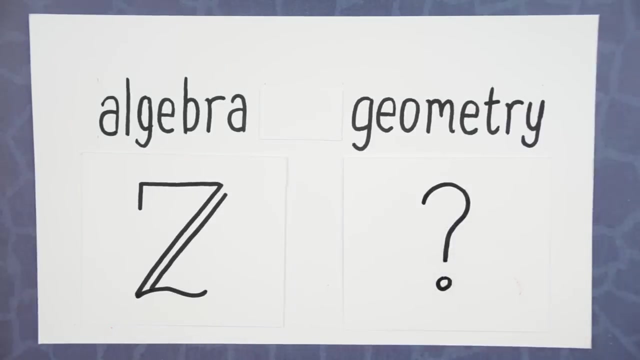 of rings. but can we reverse this procedure? what if you take any old ring like z, the ring of integers? is there a geometric object that corresponds to it? can we view z as the ring of functions on some geometric object? it turns out that there is a geometric object here and it is. 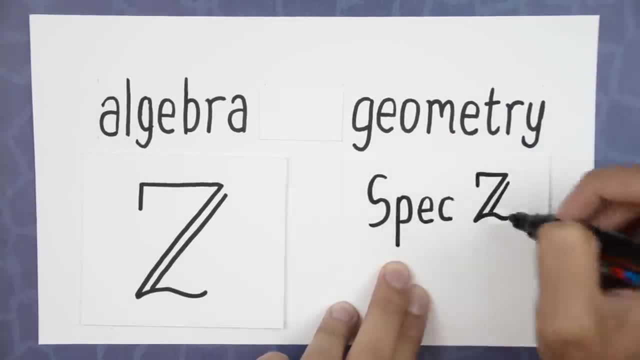 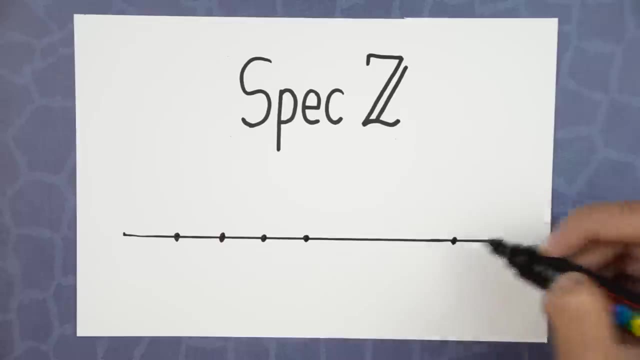 called spec z. this is an example of something called a scheme. it is a geometric realization of the ring z. this is a very advanced topic and i won't rigorously describe in this video what a scheme is, but i can draw a picture of spec z. spec z is drawn as a line and each point on this line corresponds to a prime number. 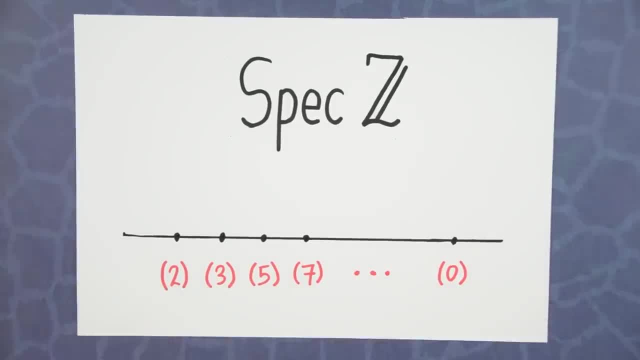 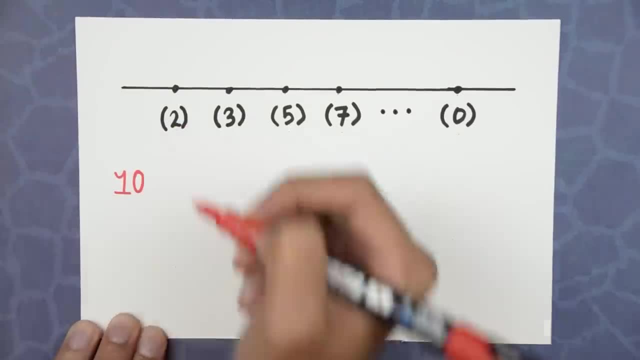 and there is one point corresponding to zero. well, how do you view integers as functions on the space? well, if i give you an integer, like, say, 10, and i ask you to evaluate it at a point on the space like 2, tell me the remainder of 10 after division by 2. so the function 10 returns the value 0 at 2. 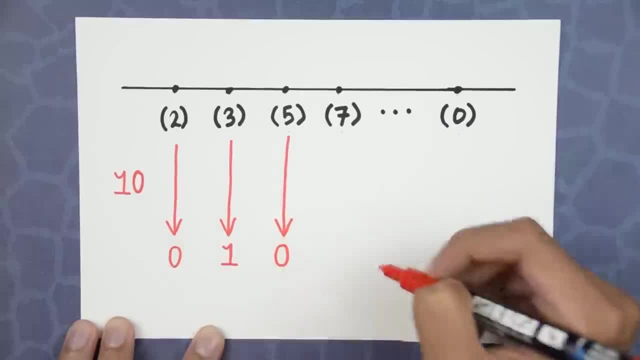 it returns the value 1 at 3.. 3, the value 0 at 5, 3 at 7 and so on, and at this mysterious point 0, it returns itself. this seems really bizarre. why on earth would we do this? it suffices to say that it turns out to 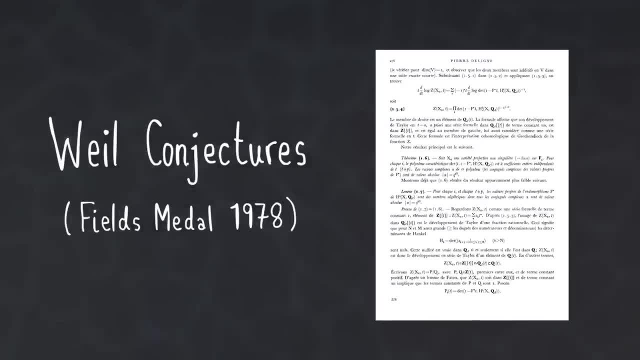 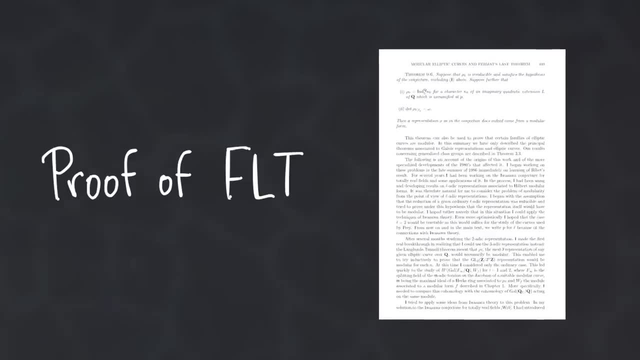 be incredibly useful. for instance, several key results in modern number theory make heavy use of algebraic geometry and the notion of a scheme. the proof of fermat's last theorem uses some very non-trivial ring theory that is motivated by gmx and algebraic geometry and the notion of a scheme. 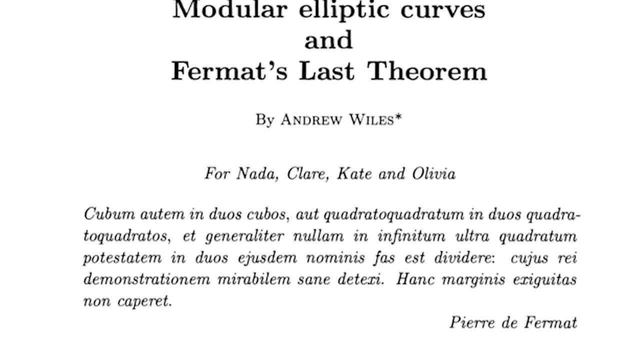 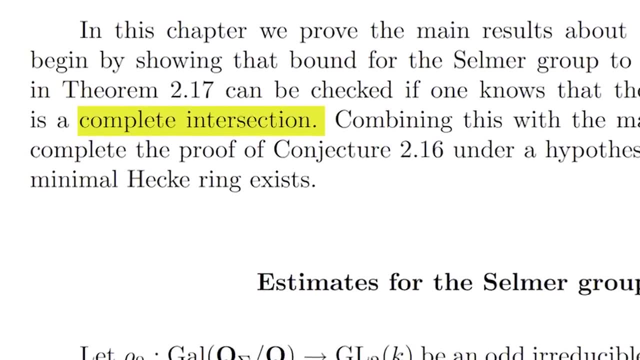 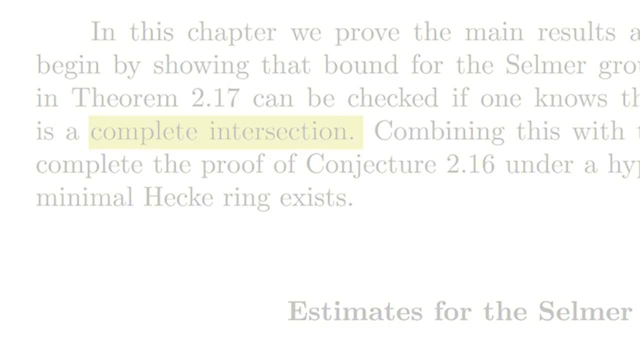 motivated by geometric considerations, An important ingredient of the proof required showing that certain rings are quote-unquote, complete intersections. Now, what that is is besides the point, but it's an algebraic property that's motivated by geometry. So that's all for the math. 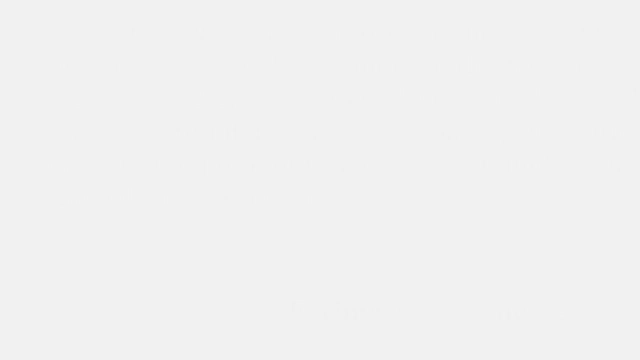 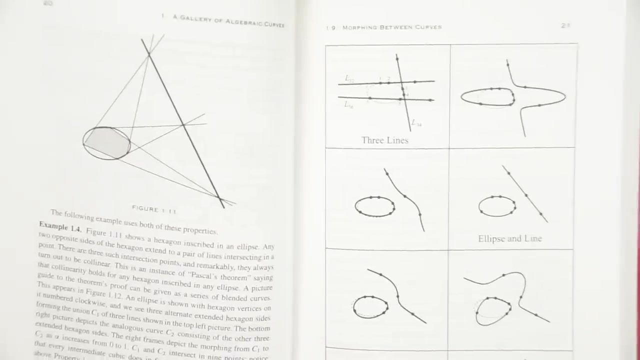 portion of this video. I'll end off by listing some resources that you can use to learn algebraic geometry in some more detail. A really good starting point is the book A Guide to Plain Algebraic Curves written by Keith Kendig. It's written in a really elementary style and has lots. 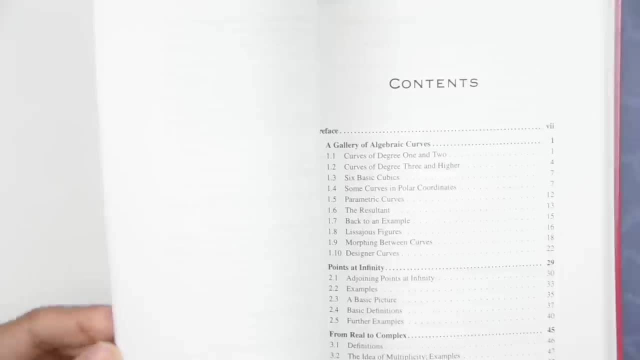 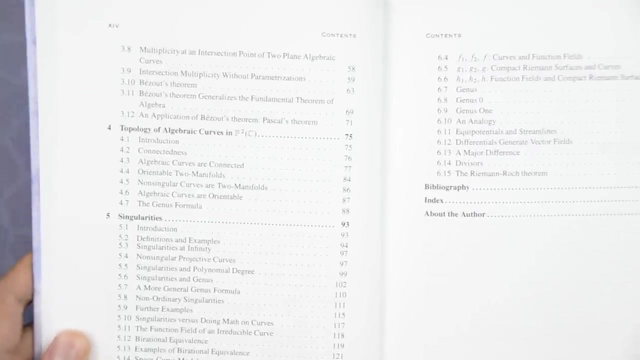 of really captivating diagrams throughout. If you look at the table of contents, it starts off with a lot of examples that require only elementary- high school level algebra to understand, but by the end it actually gets to some pretty deep theorems in algebraic geometry. 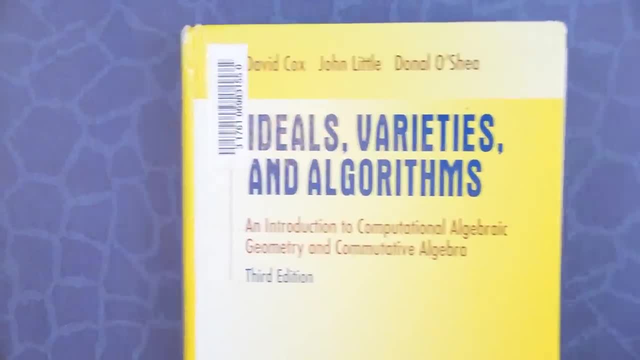 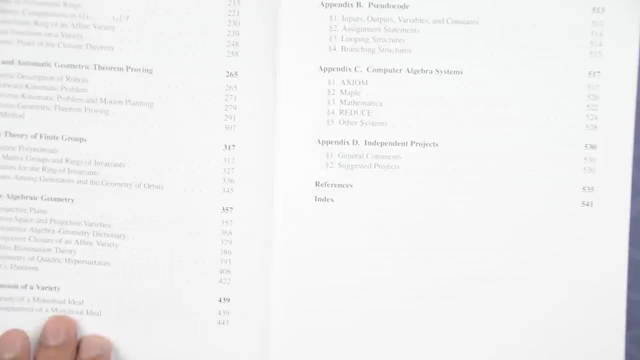 If you'd like to learn the subject in a bit more detail, using more ring theory and abstract algebra. a great book is Ideals, Varieties and Algorithms. The great thing about the book is that it doesn't assume any knowledge of abstract algebra and teaches everything from.